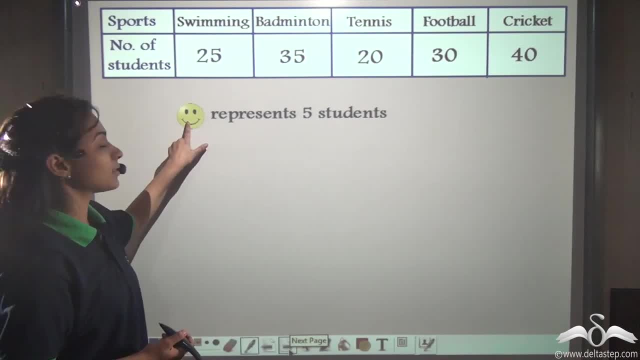 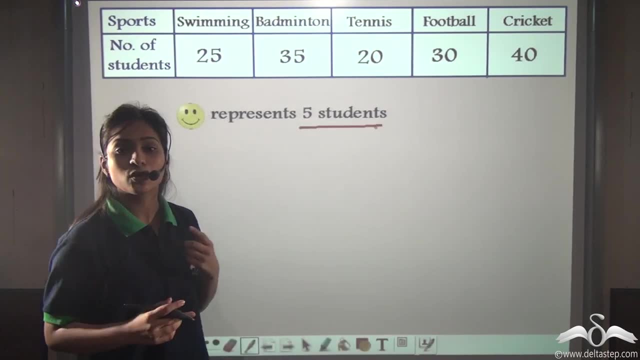 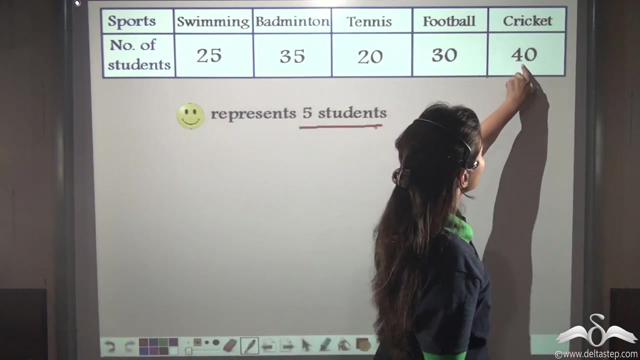 Now I am taking the symbol of a smiley and I say that one smiley represents five students. Now, why five students? Why not one student? Well, you can see that in the data given we have the number ranging from twenty to forty, So to represent the data of forty students. 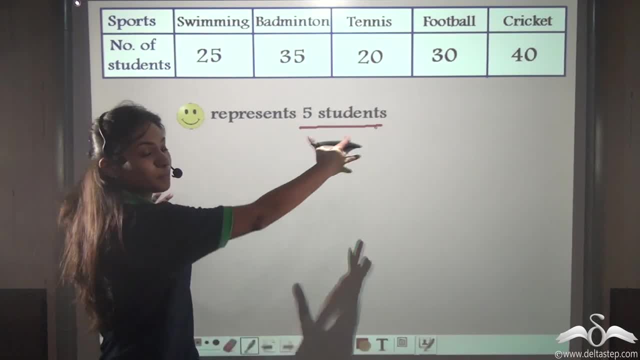 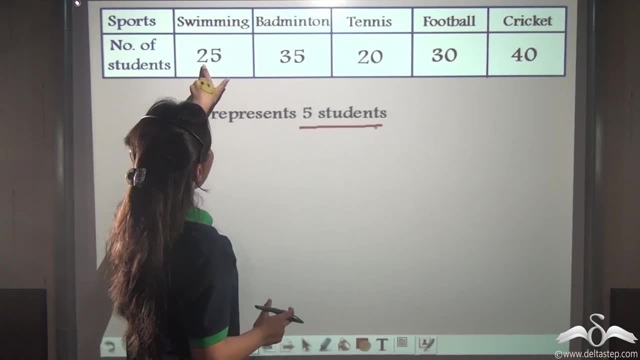 we need to make forty smileys in a row. Now. that would take a lot of space. Now we do not have so much of space, So what we will do is you can see that The data given, all the numbers here, are multiples of five. So what we are doing is we are taking. 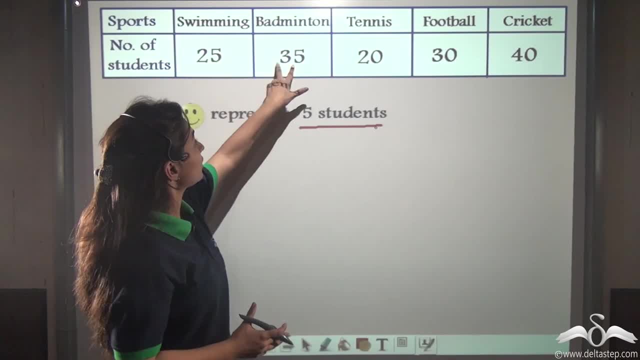 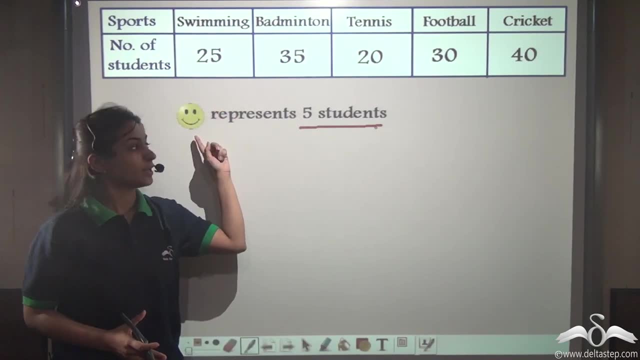 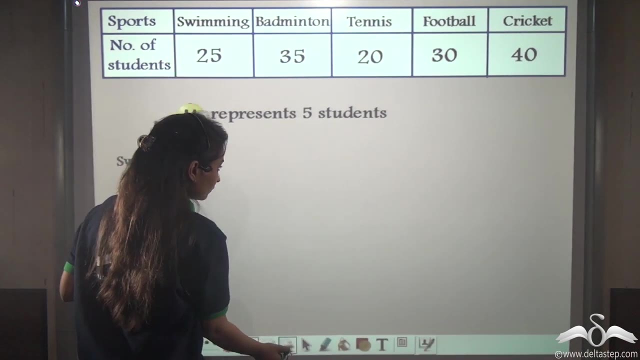 one smiley to represent five students. So, as all they are multiples of five, they are easily divisible by five and we can denote the data in the way of one smiley, which is representing five students. So what we will do is we start with swimming. So can you tell. 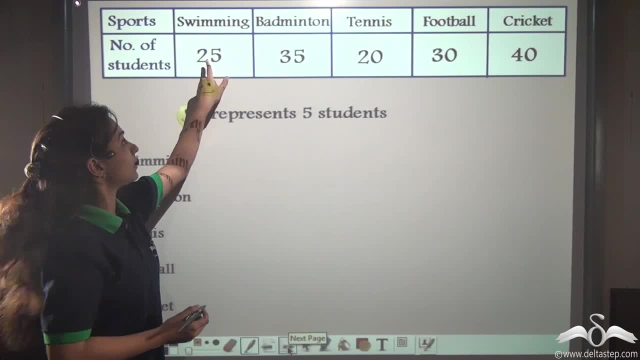 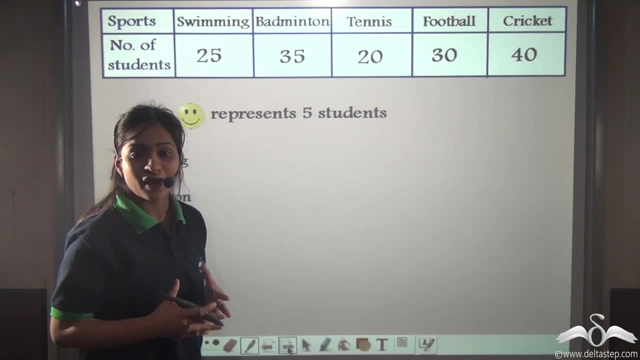 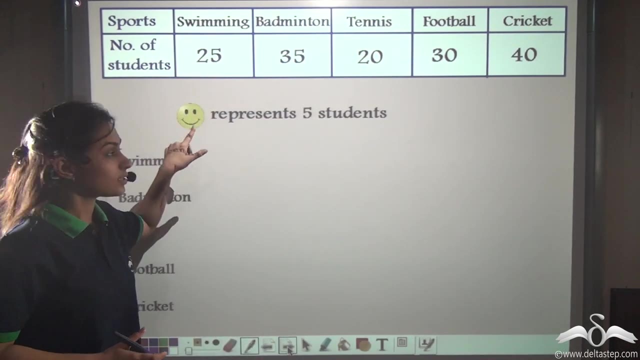 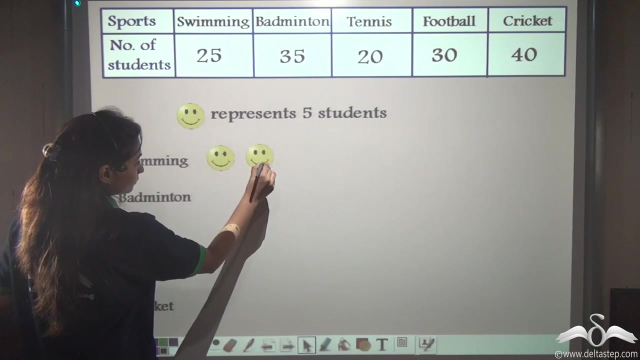 me how many smileys represent the data given for swimming? Twenty-five students. If one smiley represents five students, Well, twenty-five divided by five is five. So if one smiley represents five students, five smileys will represent twenty-five students. So let us denote the data given for swimming with five smileys. 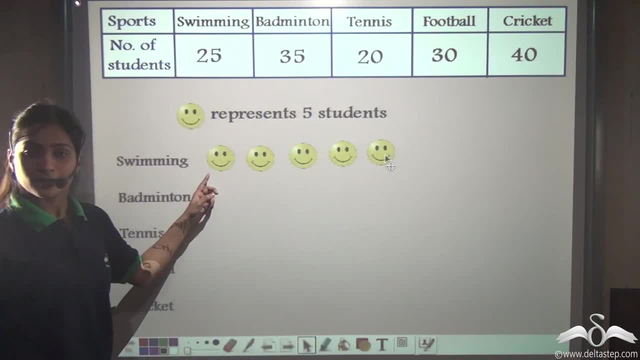 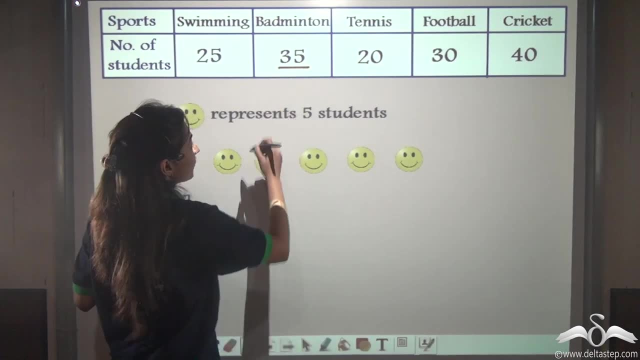 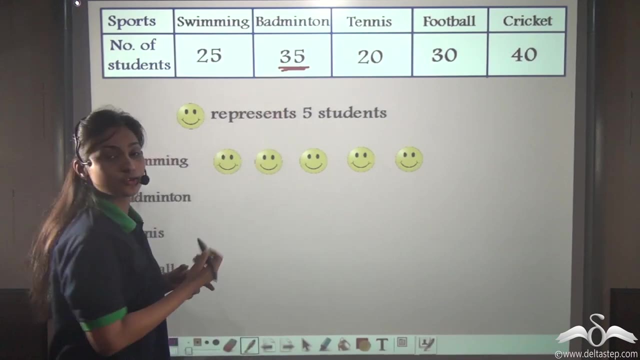 Right. Next We have bad minton. Now we have been given that thirty-five students play badminton. So if one smiley represents five students, how many smileys will represent thirty-five students? Again, thirty-five divided by five, that is seven. So seven smileys will represent thirty-five students which go for. 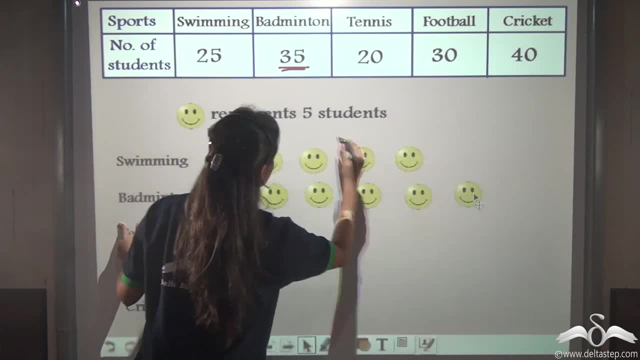 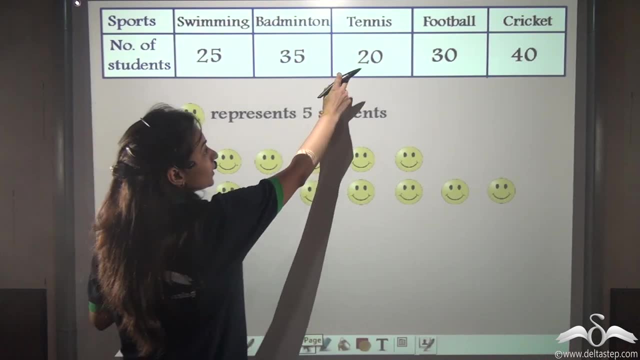 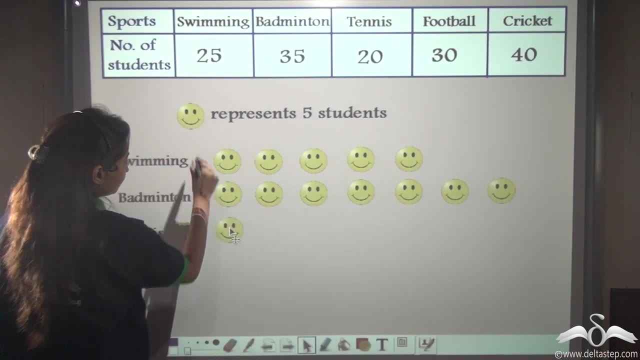 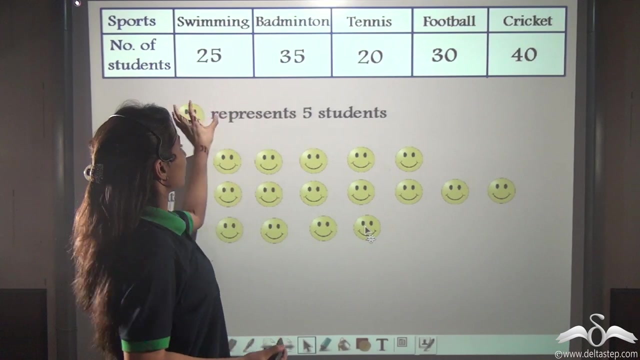 badminton. There we go. Next we have tennis. Now twenty students play tennis, So twenty divided by five: four, So four smileys will denote students going for tennis. Now, whenever you are writing such things, that one symbol represents more than one student, 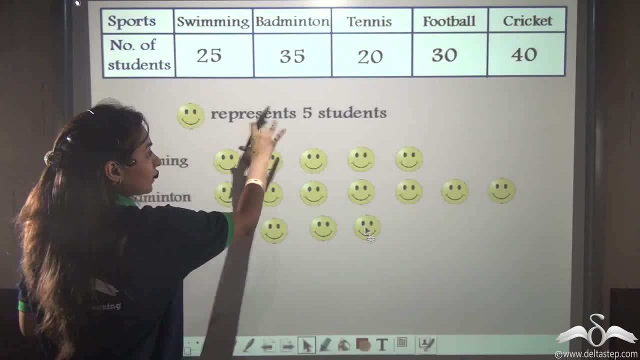 or more than one given data, you must always write it down or make a note of it so that the teacher can understand what you want to depict. Next, we have tennis. Now twenty students play tennis, So twenty divided by five, four, So four smileys will denote students going for tennis. Now, whenever you are writing such things that one symbol represents more than one student or more than one given data, you must always write it down or make a note of it so that the teacher can understand what you want to depict. 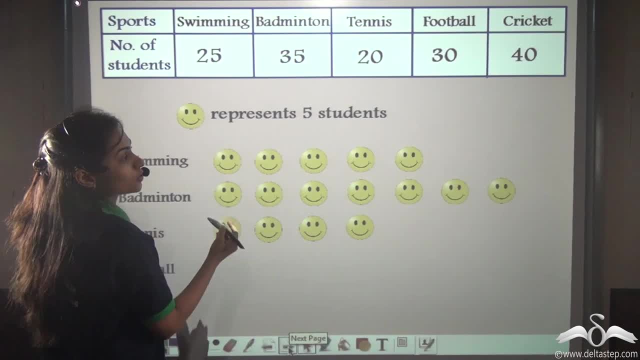 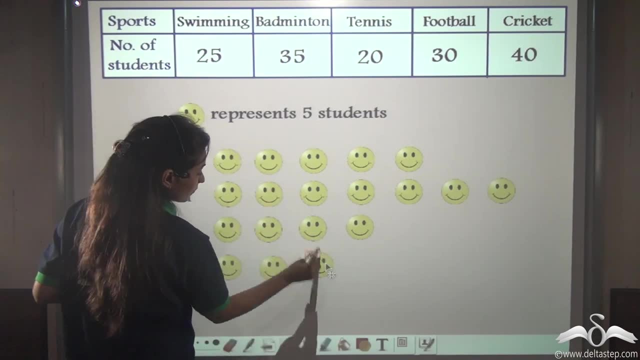 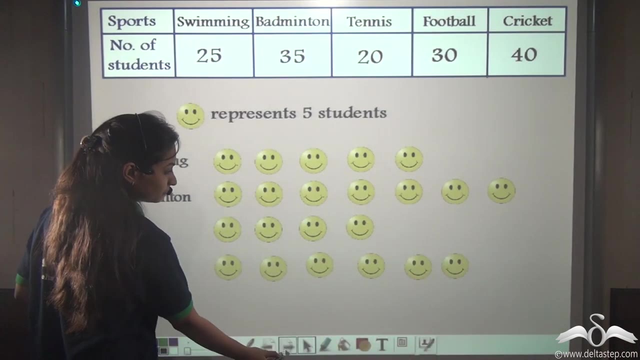 Next we have football: 30 students, 30 divided by 5, 6,, so 6 smileys for football. Next cricket: now 40 students play cricket, so 40 divided by 5, 8,, so 8 smileys for cricket. 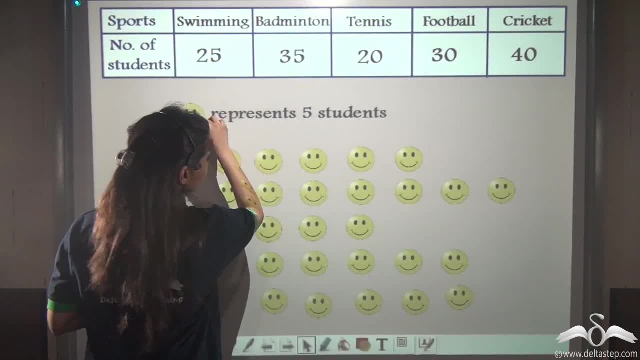 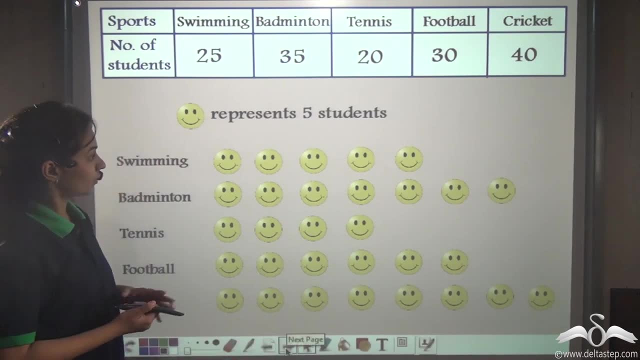 So there, we have completed our pictograph, right? So this is how you make a pictograph. Now, what I was doing, I was copying all these smileys. Now suppose you are drawing symbols. you can just draw those symbols instead of these smileys. 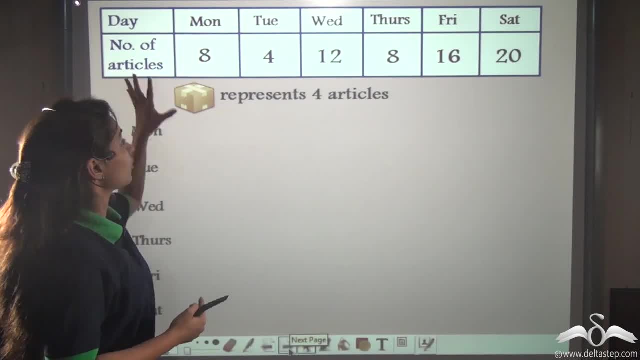 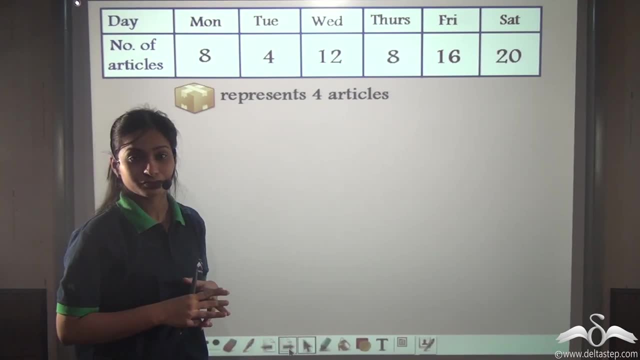 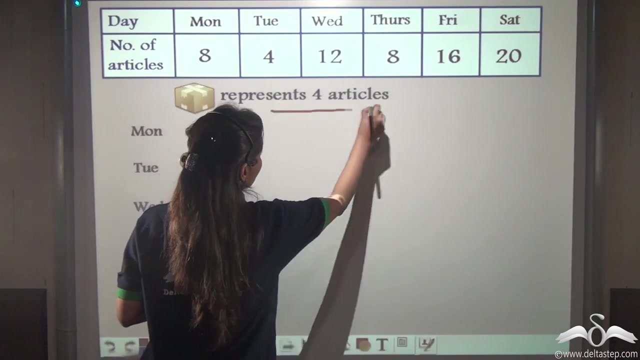 Now I have given you some other data as well. Now these are the data of number of articles sold by a shop from Monday to Friday, From Monday to Saturday. Now make a pictograph for this data. Well, here I have taken the symbol of this box to represent 4 articles. 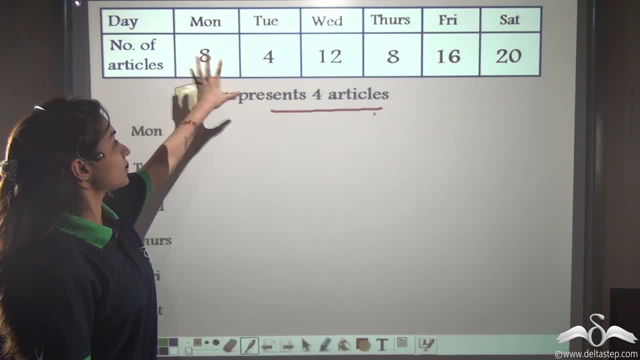 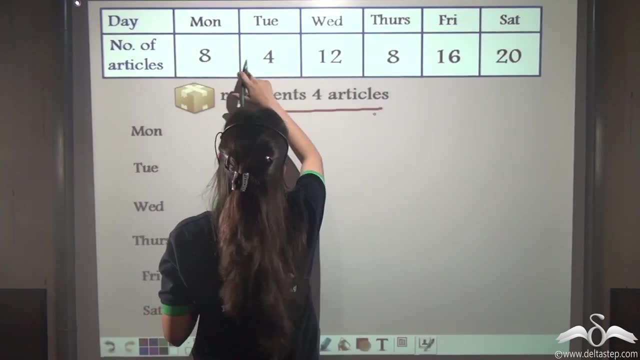 Now, why 4 articles? Well, I can also denote this data, taking one symbol to represent one article. But here I can see that all the numbers here- 8,, 4, 12, 8,, 16,, 20- are multiples of 4 and 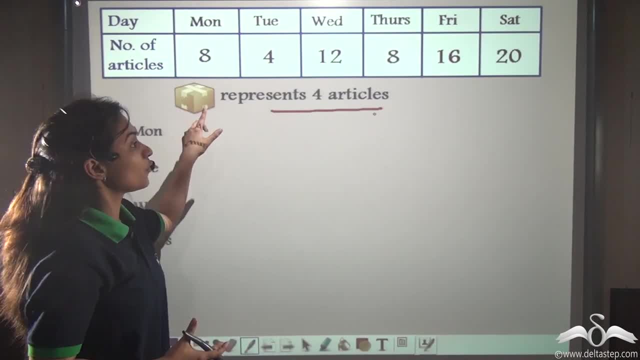 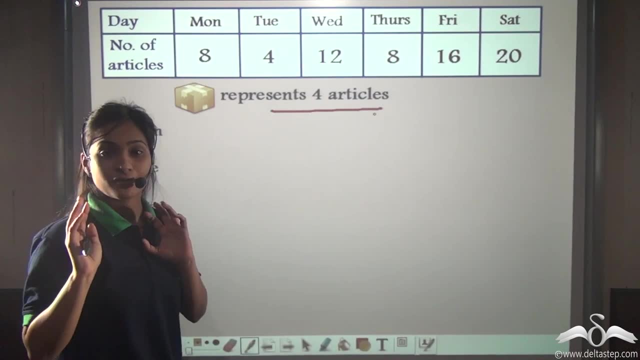 they are also multiples of 2.. So, if you want, you can take a symbol Which represents 2 articles as well as 4 articles. So let us start making pictograph for this. Now you are familiar how to make a pictograph, so do it on your own. 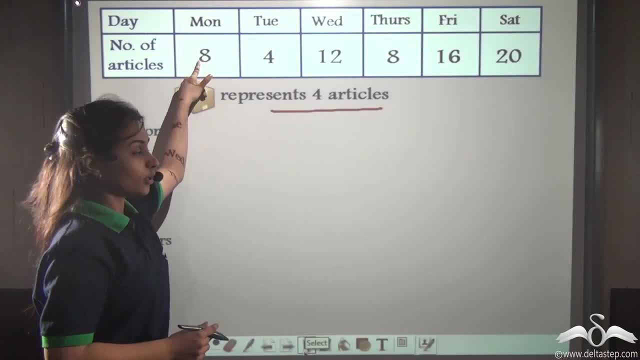 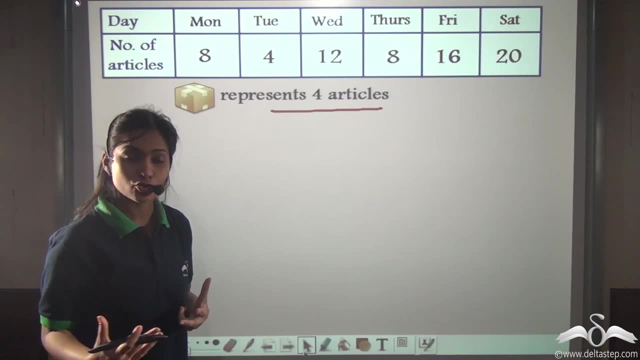 Let us do it together. On Monday, 8 articles were sold. Now one box represents 4 articles. So how many boxes will denote 8 articles? 8 by 4, that is 2, so 2 boxes denote 8 articles. 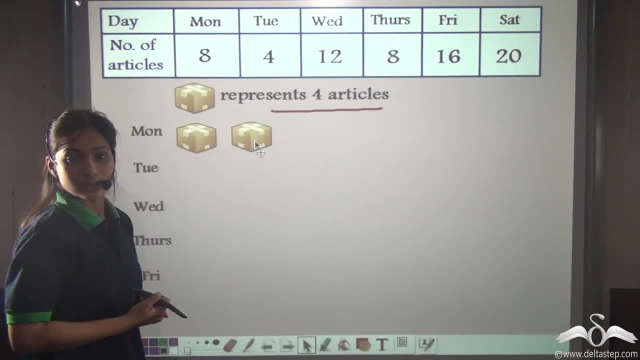 that were sold on Monday. Similarly for Tuesday: 4 articles. Now one box denote 4 articles, so only one box for Tuesday. Similarly Wednesday: 12,. so 12 divided by 4, 3, so 3 boxes for Wednesday. 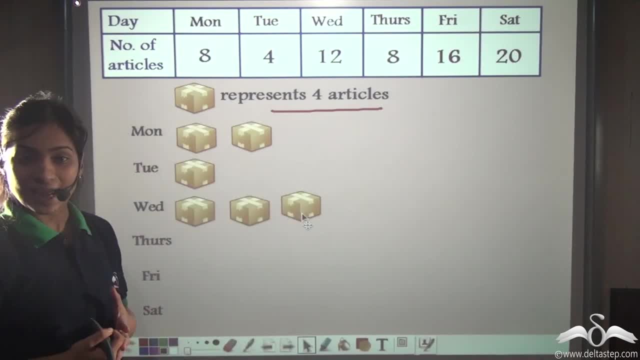 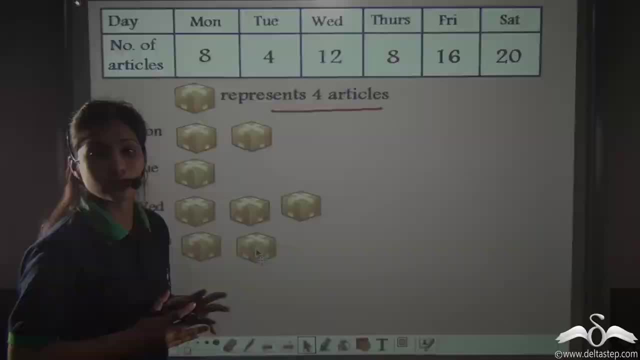 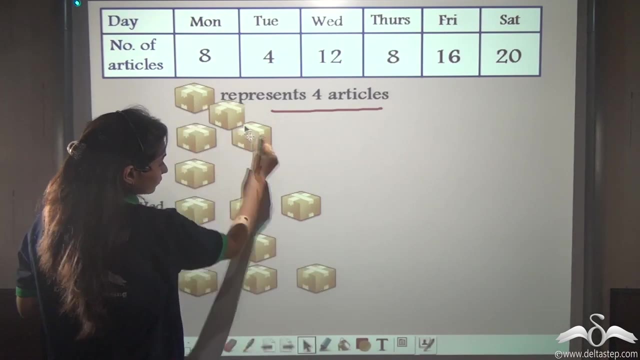 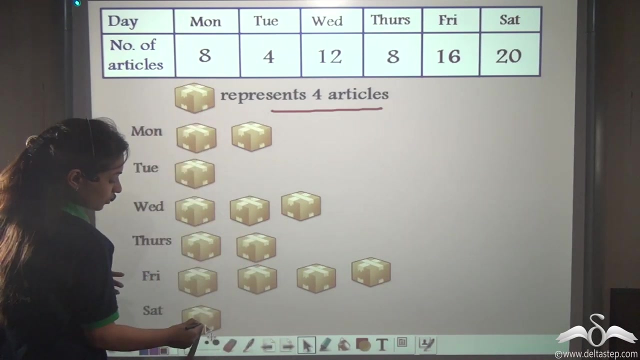 Now on Thursday: 8, so 2 boxes for Thursday. Similarly for Friday: 16, so 16 divided by 4, 4, so 4 boxes for Friday And last. we have 20 articles on Saturday, so 20 divided by 4, that is 5, so 5 boxes for. 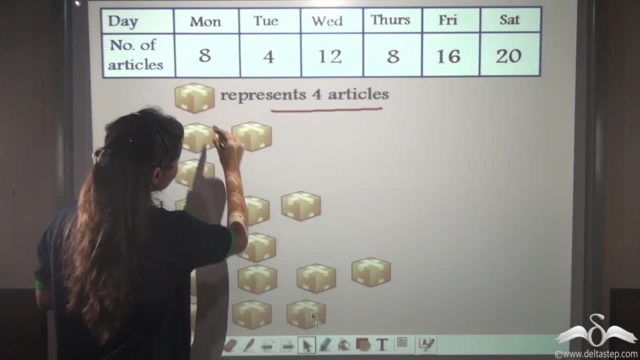 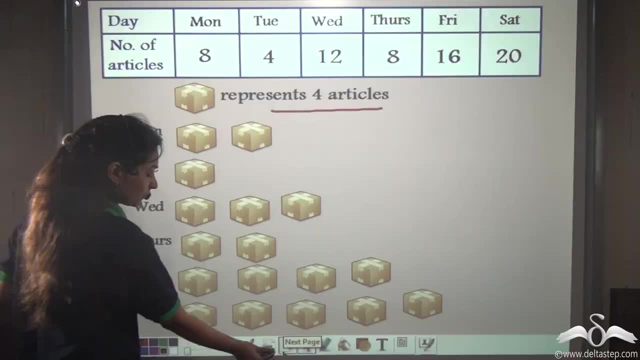 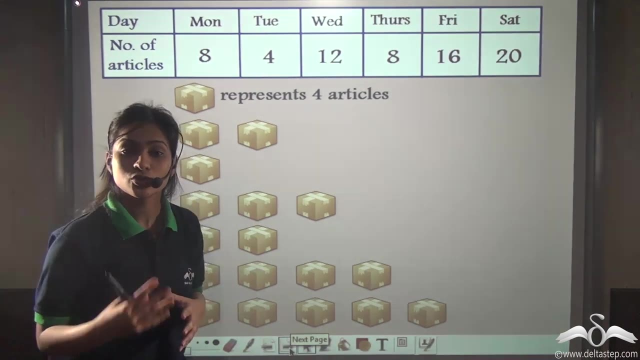 Saturday. So there we are ready with our pictograph. Now, every time, you may not have to draw the pictograph, You might be given a pictograph and you can be asked questions. So let us see what kind of questions you can be asked. 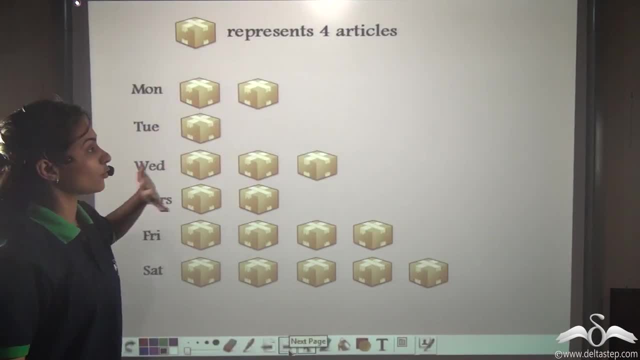 Well, suppose this is the picture, So let us see what kind of questions you can be asked. Well, suppose this is the picture, So let us see what kind of questions you can be asked. So let us see what kind of questions you can be asked. 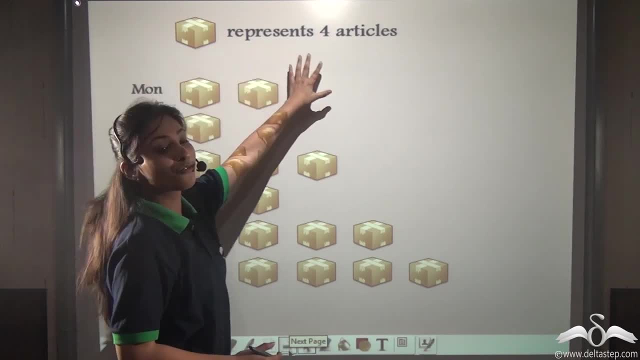 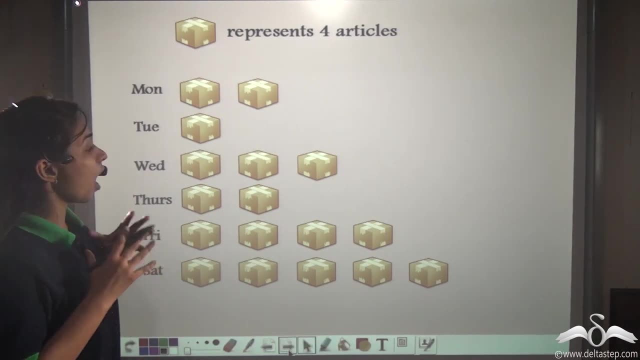 So, first of all, a number of the pictograph that you have already made now is given to you. Now you have been told that one box represents 4 articles and this is the pictograph given to you. First of all, can you tell me from the pictograph itself how many articles were sold on, say, 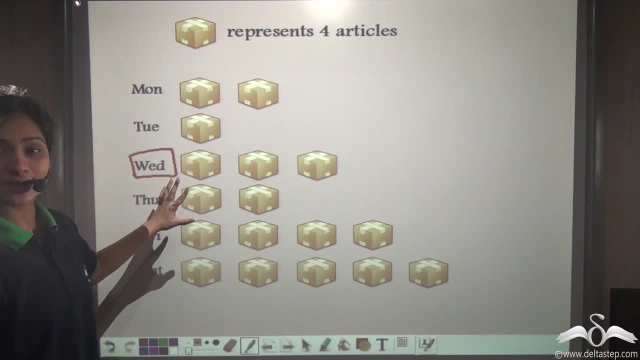 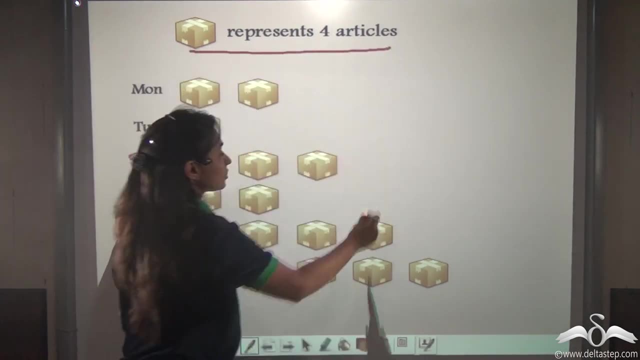 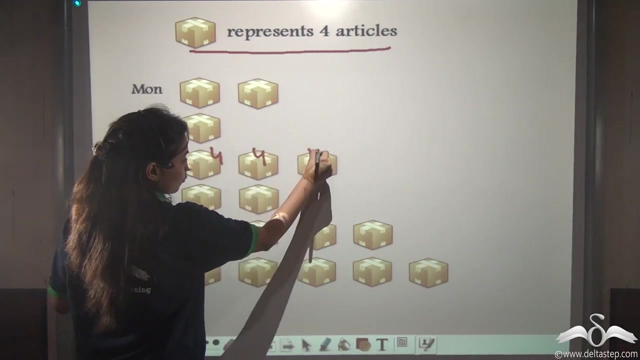 Wednesday. Now you can see three boxes are denoting articles sold on Wednesday and one box represents four articles. So tell me the number of articles sold on Wednesday. Well, 4 plus 4 plus 4, that means 4 into 3, that is 12 articles, right? 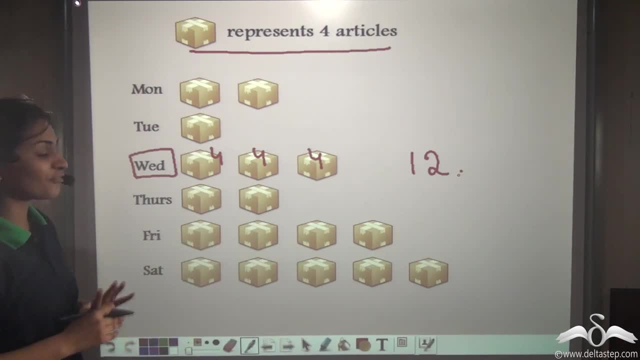 Now tell me the number of articles sold on Friday Again: 1,, 2,, 3,, 4, 4 boxes. 1 box denotes 4 articles, 4 into 4, 16.. Now tell me, according to the pictograph, which day do you think were the least number of articles sold? 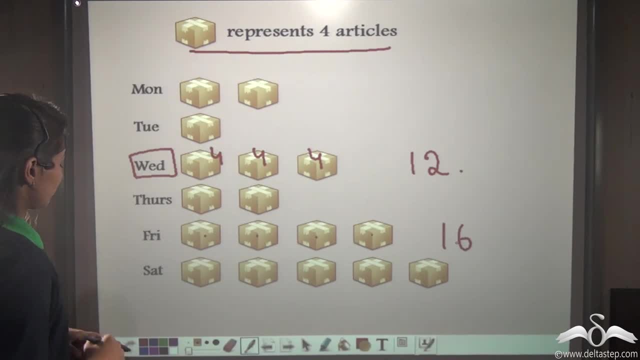 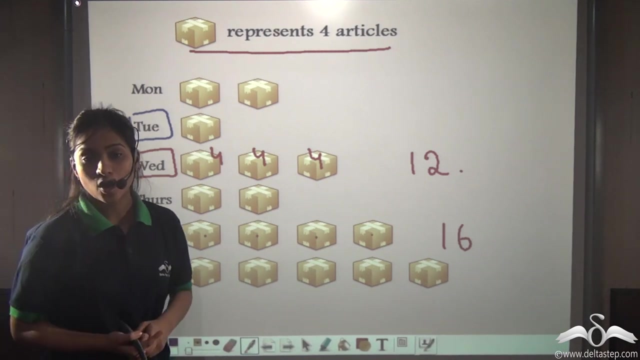 Have a look. Well, the least number of articles were sold on Tuesday, because only Tuesday is the day where only 1 box is sold. Otherwise all have more than 1.. Next, tell me on which day were most of the articles sold.